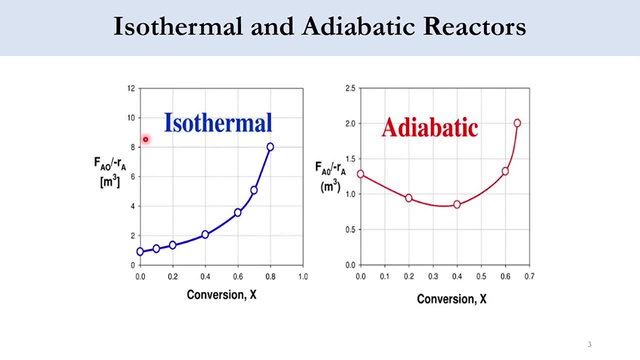 But before going to that we will first review the isothermal and adiabatic reactor strand. And at this point we had ended the previous lecture That for isothermal system, with the increase in conversion the value of FA0 over minus RA increases, And we had said that for such type of systems we prefer PFR over the CSTRs. 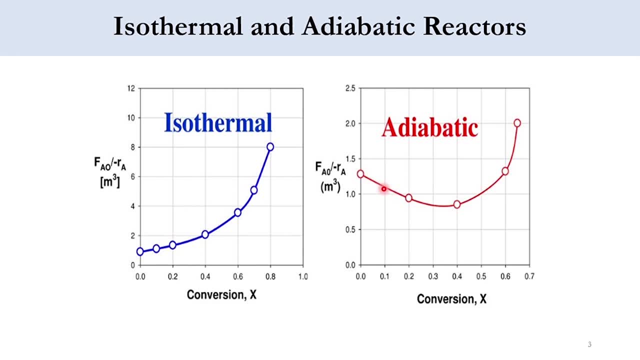 In this adiabatic system we had seen that first the value of FA0 over minus RA decreases and then it has increased. And we have seen that initially the rate of reaction is higher And as the time passes, as the conversion increases, the value of rate of reaction increases. 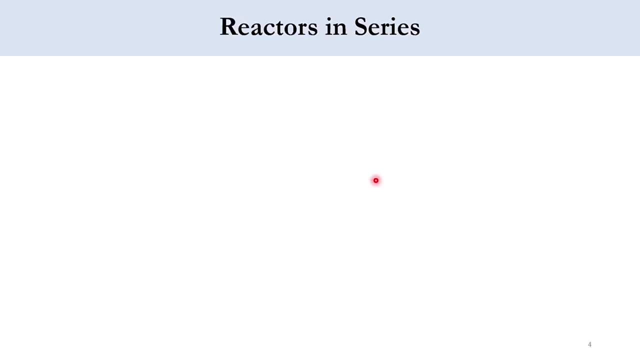 So, accordingly, we had observed these strands. Now, starting with the reactors in series, exit stream of one reactor will be definitely inlet stream for the other reactor. The outlet of first reactor will be the inlet of second reactor. The outlet of second reactor will be the inlet of third reactor. 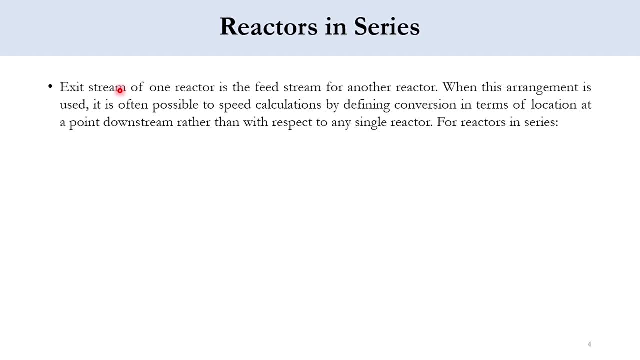 So accordingly, we have to define the conversion, that how much conversion is achieved for the species A. So accordingly, the formula will be that if there are I number of reactors, There will be a reaction of. I is equal to total moles of A reacted up to point I, divided by moles of A fed to the first reactor. 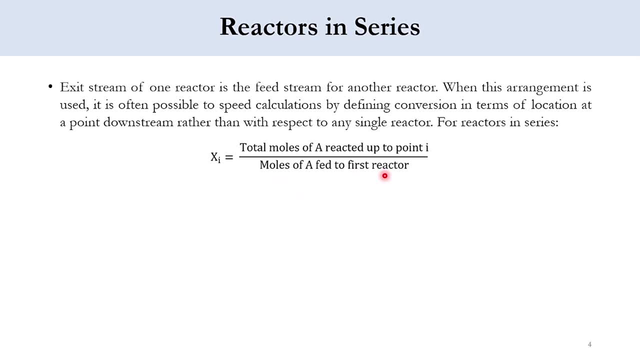 Initial flow rate of the A and the exit, the final flow rate which is, for example, if there are three reactors in the system, we say that we will be calculating the X3. And that X3 will be the conversion which will be obtained in the third reactor. 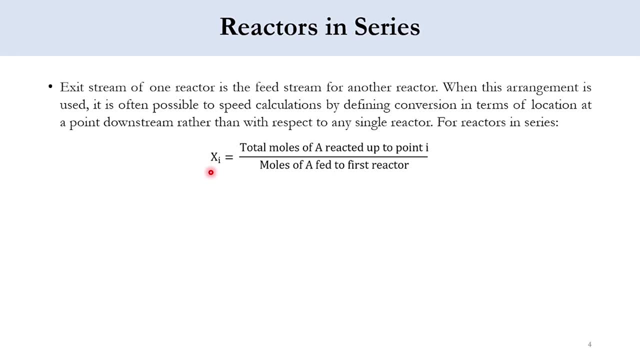 And accordingly the value or the molar flow rate of A at the outlet of the third reactor will be considered. so accordingly it will be FA0, the initial flow rate minus the final flow rate, which is FA3. so accordingly we will see how many moles have reacted in the system divided by moles. 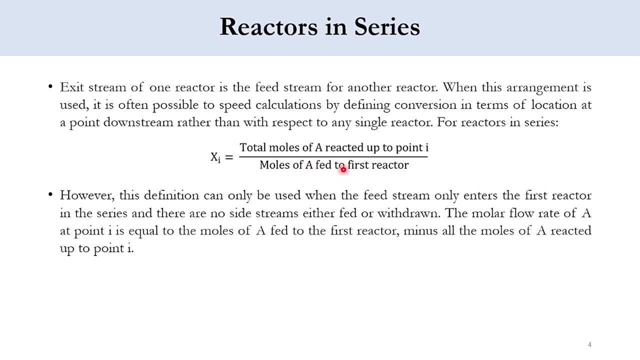 of a fed to the reactor. However, there is a condition: that it could only be used when there are no side streams in the system, either feed or withdrawn. So accordingly we will write the value as FAi is equal to FA0 minus FA0 into Xi, which means that if it is for the first reactor, FA1. 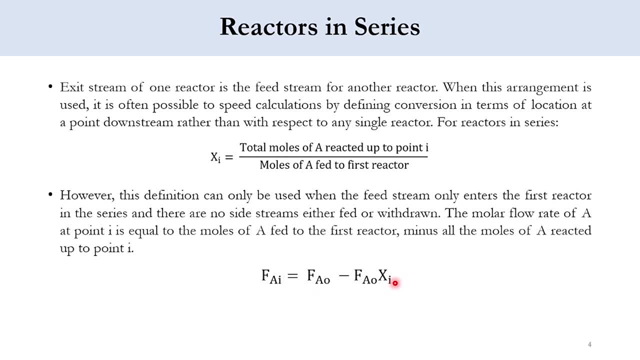 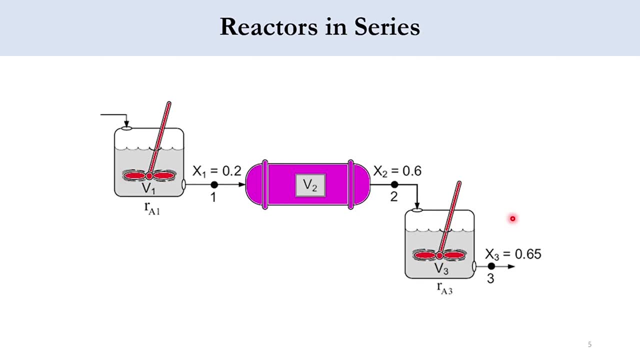 is equal to FA0 minus FA0 into X1.. For second reactor, FA2 is equal to FA0 minus FA0 X2.. Now let's move to an example and see how this can work. There are three reactors in series. first is CSTR. 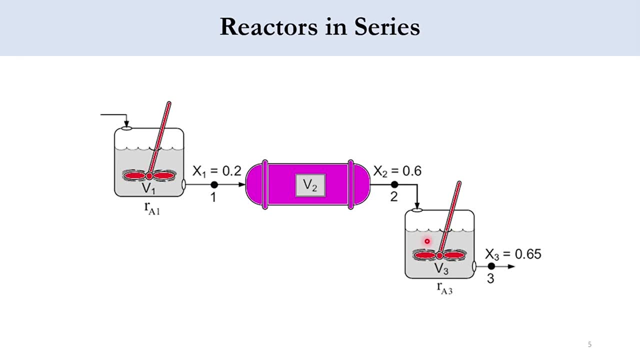 second is PFR and third is again CSTR, Volume V1, V2 and V3. respectively. So this is the feed at the first point in the first reactor, which is FA0. Here it will be FA1, FA2 and FA3.. In the first reactor, 20% conversion takes place At the end of second. 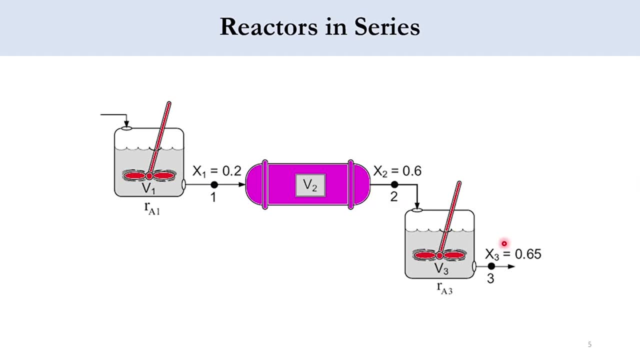 reactor, 60% conversion takes place and finally, 65% conversion takes place. So what we will need to do to find the overall conversion, obviously we will take this FA0 and this FA3 to find out the total or overall conversion. We need to calculate the conversion at each point, like 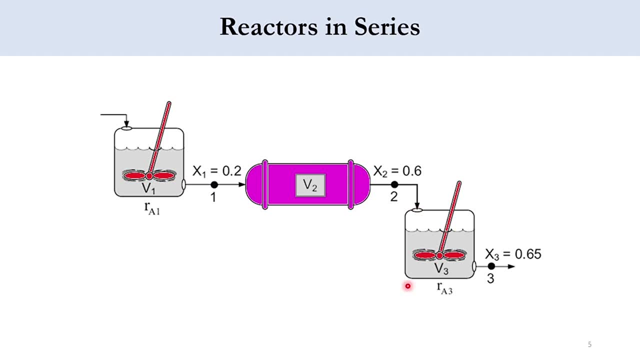 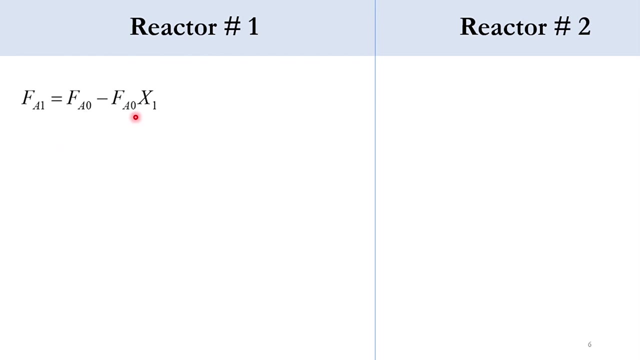 in the first reactor, in the second reactor, in the third reactor. Now, since we are given the conversions, what we need to do we need to calculate the volumes of this reactor, which is V1, V2 and V3. The general mole balance will be: FA1 is equal to FA0 minus FA0 X1. Obviously, we have seen this. 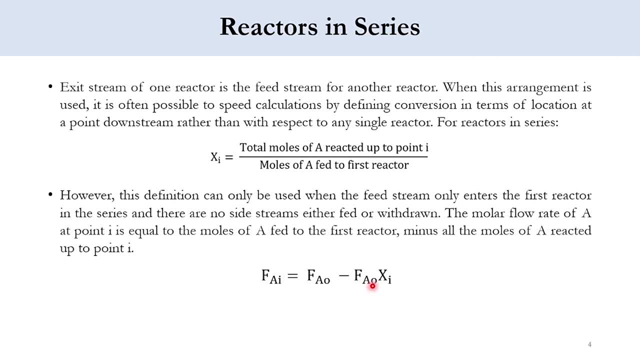 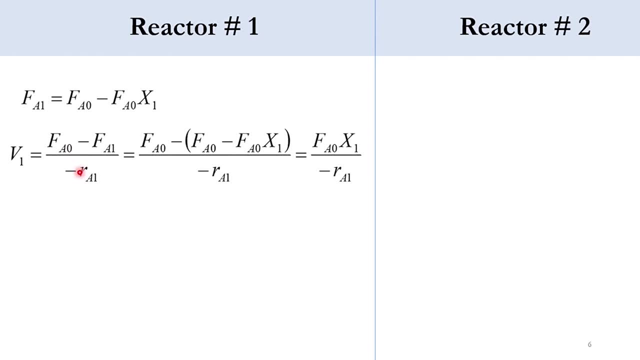 equation: FAi is equal to FA0 minus FA0 Xi. So FA1 is equal to FA0 minus FA0 X1.. Accordingly, V1 is equal to FA0 minus FA1 over minus RA1.. FA1 is equal to FA0 minus FA0 X1.. So according to this FA0, FA0 will cancel out and we get. 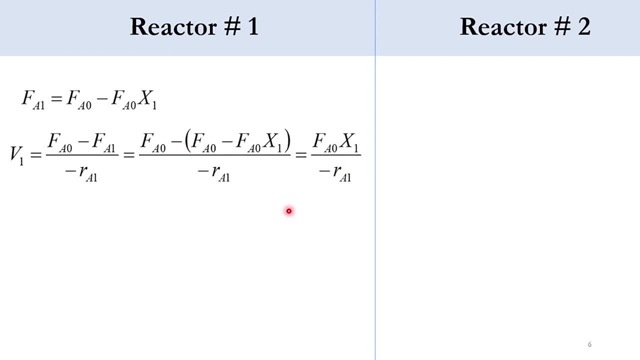 FA0, X1 over minus RA1, which is represented by this region up to X1 for the adiabatic system. Now second one is the BFR. So accordingly, V2 is equal to integral X1 to X2. FA0 over minus. 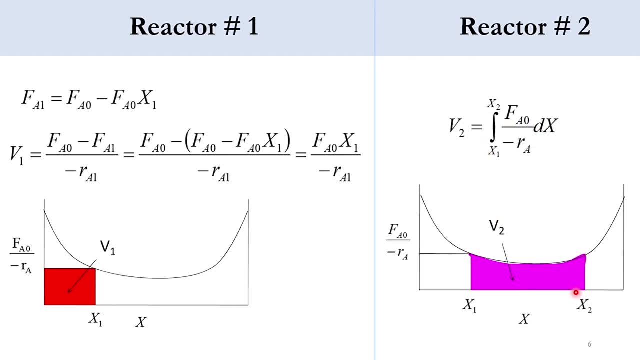 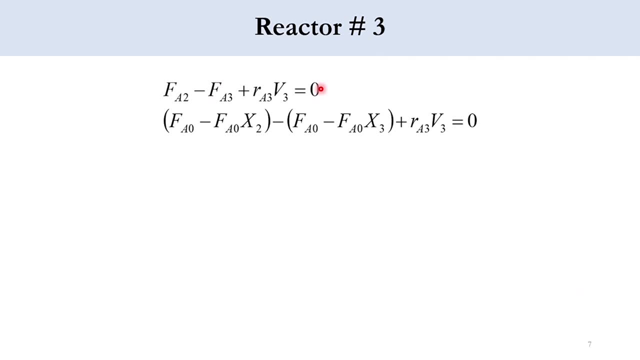 RA into dx and it is represented by this shaded region. For the third reactor, again, we will first apply that equation that FA2 minus FA3 plus RA3 V3 is equal to zero. This is the general mole balance equation and for FA2 it will be FA0 minus FA0 X2.. For FA3 it will be FA0. 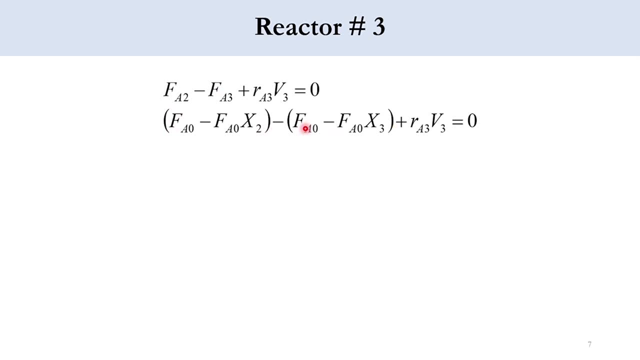 minus FA0 X3. So this FA0 will cancel out with this FA0. Accordingly we will be left as FA0 X3 minus FA0. X2 is equal to minus RA3 into V3. And accordingly, on rearranging we get V3 is equal to. 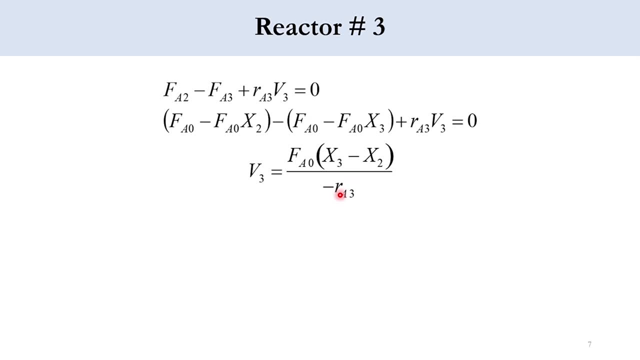 FA0, X3 minus X2 over minus RA3 and it is represented by this region. So you can see that for the three reactors we have derived the equations. Obviously, for PFR there was no need to derivation. the equation was straightforward, we had to just change the limits. But in this case, in the CSTR, 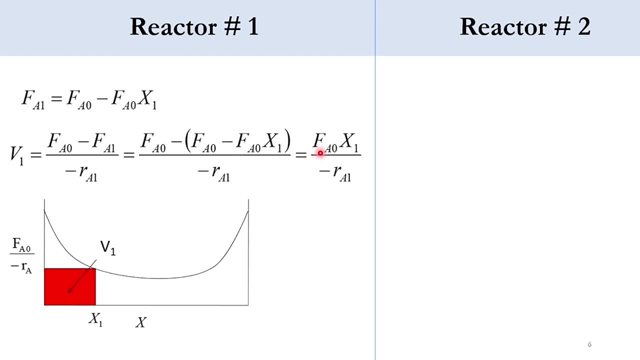 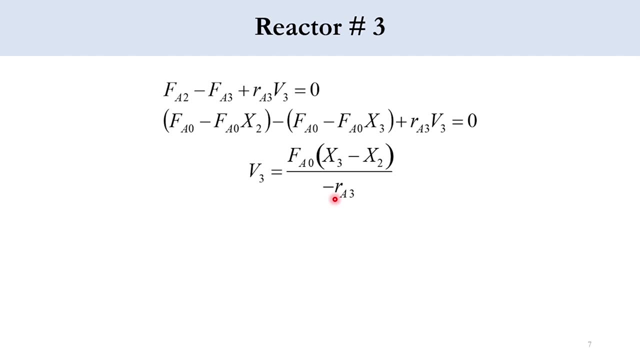 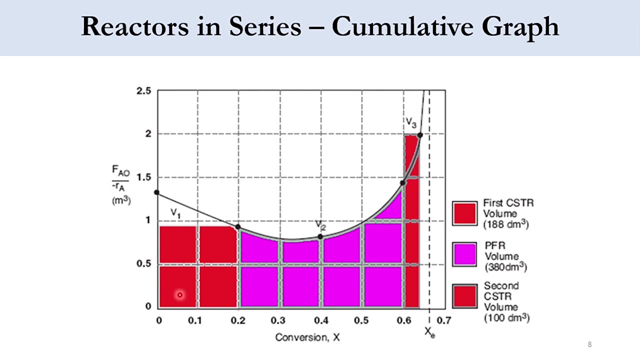 for the first reactor it was FA0- X1 over minus RA1 and for the third reactor it was V3- FA0- X3 minus X2 over rate of reaction for that particular system. So accordingly we get this overall trend for the adiabatic system. Now you can see here that this region for 20 percent represents for 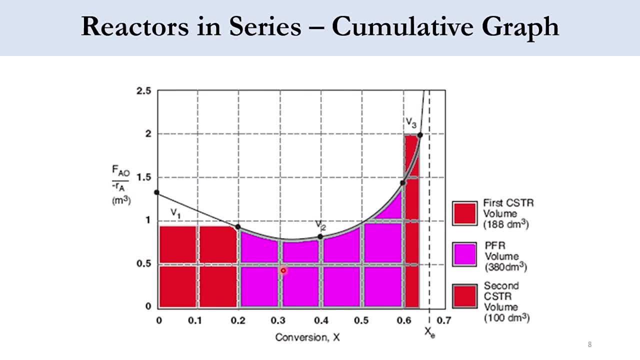 PFR. For 20 to 60 percent it represents the PFR, and for 60 to 65 percent it represents again the CSTR. Now my question is: if we install PFR first, then what will happen? PFR covers the area under: 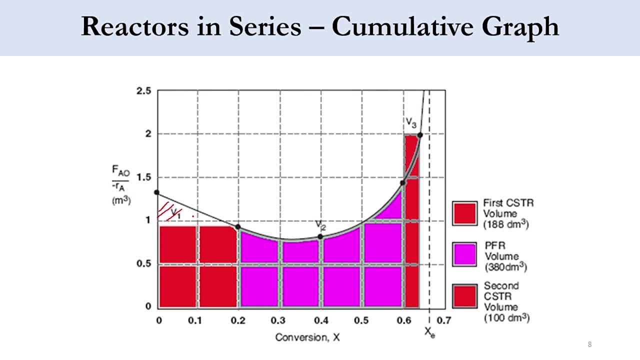 the curve. while this point, this region is empty. here, This region is not occupied. It means that for the adiabatic system we have to check whether CSTR is preferable or PFR. Initially, you can see that here CSTR is preferable in comparison to the PFR. Now we have to check whether CSTR is preferable or PFR. Initially, you can see that here CSTR is preferable in comparison to the PFR. 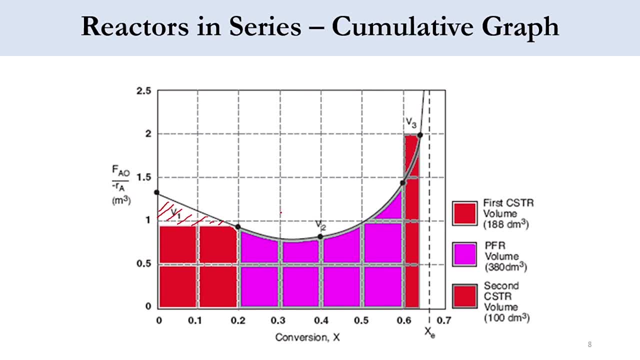 While in this region where PFR is installed, if you install the CSTR, then accordingly it will, you can see this area will be occupied or this area will be considered. So if we switch the places accordingly, we get higher volume than this base case. So accordingly, you can see that for the adiabatic, 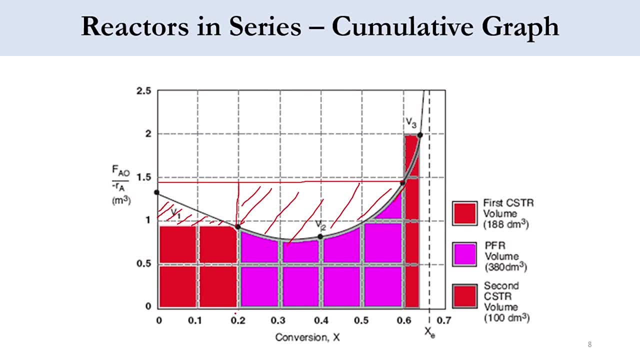 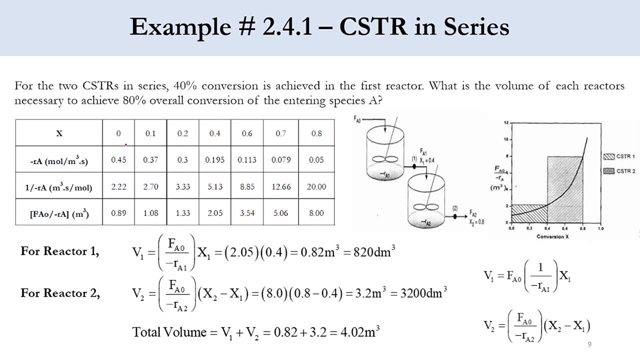 system. it is not a straightforward case as that of the isothermal system. Now let's move to the example and solve it. that we have the same example as we have solved in our previous lecture, 5 and 6, which give us the conversion of 80%. We have divided it into two reactors. First, one gives the 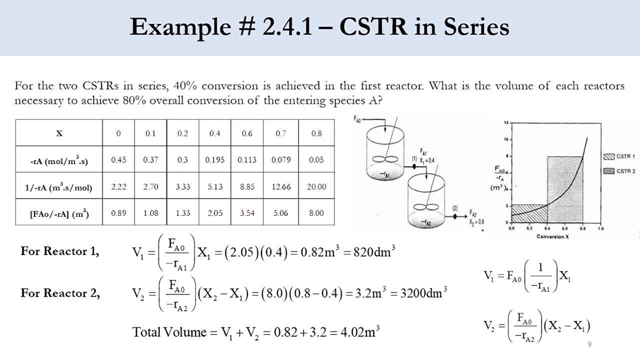 conversion of 40%, and the second one gives the conversion from 40 to 80%. So, accordingly, what we need to do? we know that V1 is equal to FA0-RA1 into X1. We have just derived that equation. Now FA0-RA1 will be required at conversion- 40%, So it will be 2.05 and X1 is 40%. 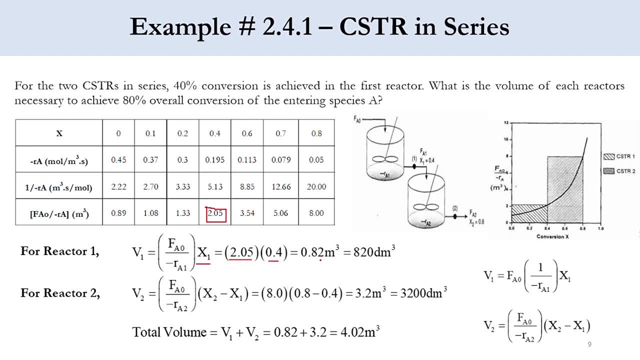 0.4. 0.05 multiplied by 0.4 gives an answer of 0.82 cubic meter or 820 cubic decimeter For second reactor. if you again apply mole balance and derive that equation, you get V2 is equal to. 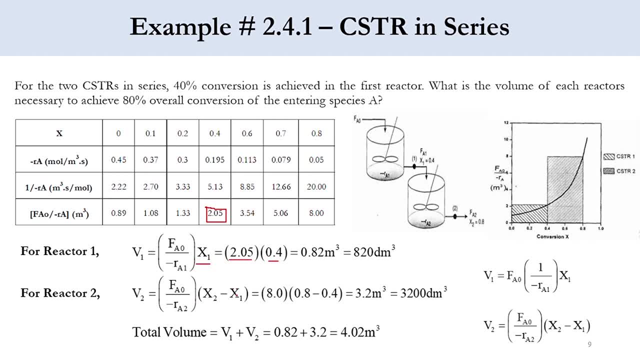 FA0-RA2- X2-X1.. For V3 it was X3-X2.. So you can see the trend that for the first reactor it will be simply FA0-RA at X1, but for the second reactor it will be X2-X1.. For third reactor will be X3-X1. 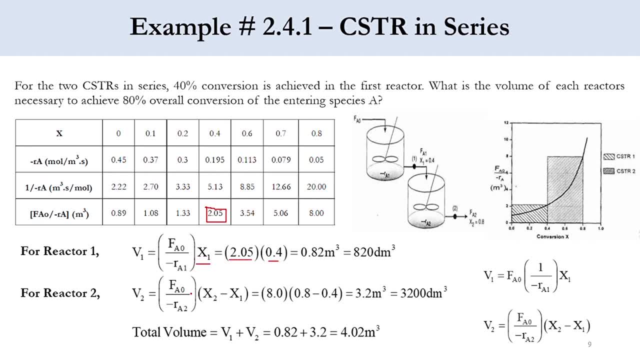 X2.. Fourth reactor will be X4-X3 according to the FA0-RA at that particular point. So X2 is 0.8, X1 is 0.4.. This FA0-RA2 at 80% corresponds to a value of 8.. So 8 multiplied by 0.8 minus 0.4.. 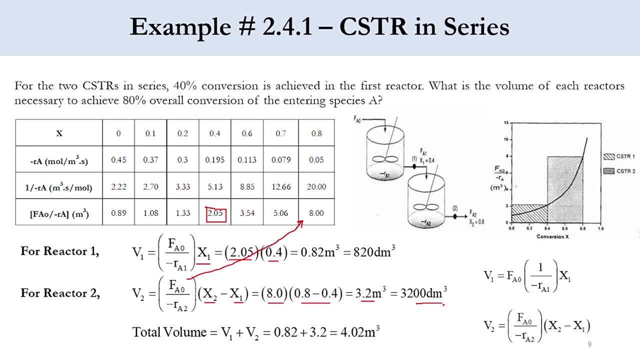 So accordingly, that will be 3.2 cubic meter or 3200 cubic decimeter. So once you sum up these two reactors volume, it will be 4.02 cubic meter. If you remember the previous reactor activity, we had calculated the volume to be 6.4 cubic meter. It was a single reactor for the same 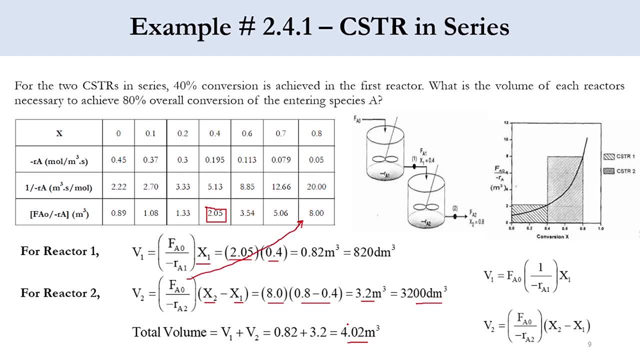 conditions, but it was for 0 to 80% conversion Here. in that case we have divided that reactor into two reactors. First one given conversion of 40%, while remaining 40 to 80% conversion was obtained in the second reactor. So you can see that the volume of the reactor is reduced. 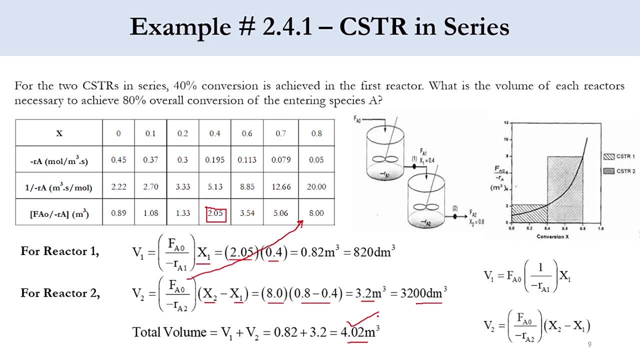 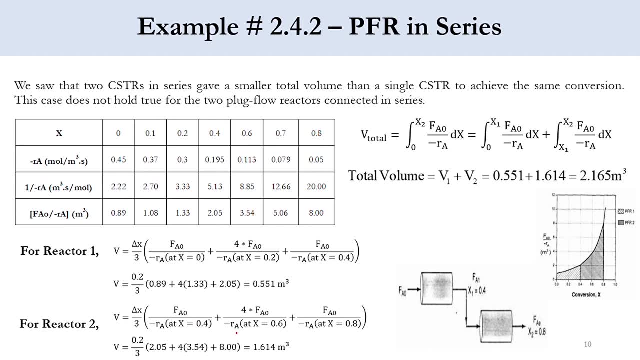 If you further divide it into more reactors, you will see the volume will decrease. Now, moving on further, we will apply here Simpson 1, third rule, and that rule states that delta X over 3, F0 plus 4, F1 plus F2.. So accordingly that will be: FA0-RA at X is equal to 0.. FA0-RA at X is equal to 0.2 because 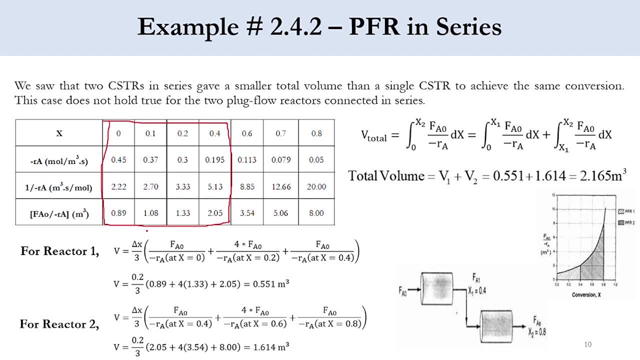 first we will take 40% conversion again, So that X, which is the step size that is calculated, final minus initial, divided by 2.. So accordingly it will be 0.2.. So FA0-RA at X is equal to 0.2 and FA0-RA. 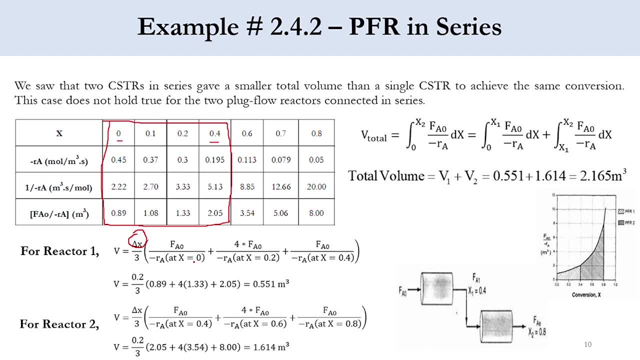 at X is equal to 0.4 for the first part. For the second part, from 40 to 80 percent conversion: 0.8 minus 0.4 divided by 2.. So again it will be 0.2.. It means 0.4. 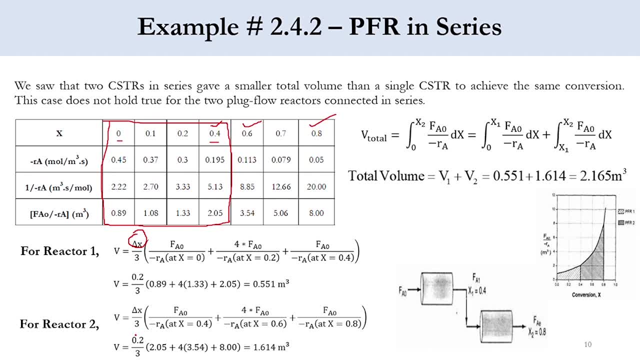 0.6 and 0.8. so accordingly, delta X over 3 FA0-RA at X is equal to 0.4, X is equal to 0.6 and X is equal to 0.8.. So this value, at X is equal to 0, corresponds to 0.89.. 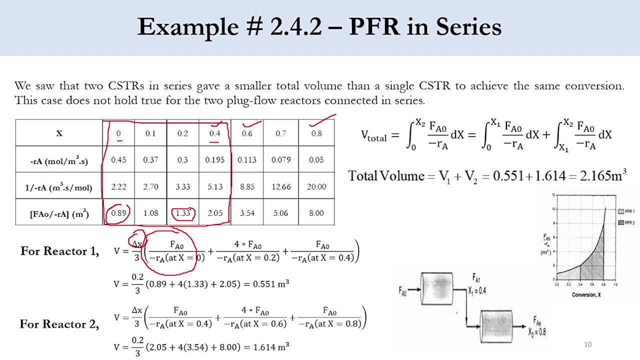 This value, at X is equal to 0.2, corresponds to this 1.33, and at X is equal to 0.4, this corresponds to 2.05. so accordingly we get a value of 0.551 cubic meter for the second reactor of pfr fa. 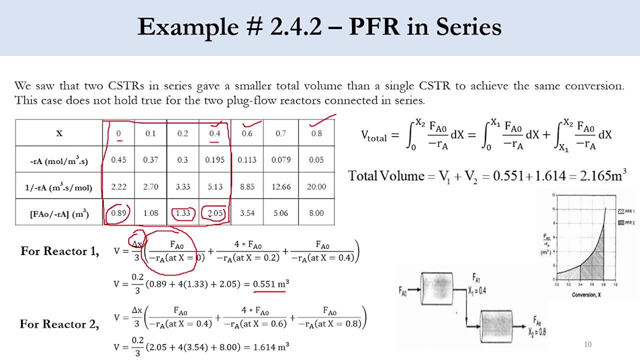 naught over minus r. a at x is equal to 0.4, corresponds to 2.05, next one 3.54 and next one 8, so accordingly we get an answer of 1.614 cubic meter. so once we add up these two we get an volume. 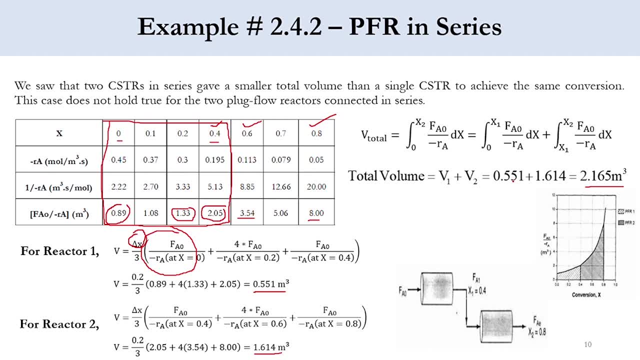 of 2.165 cubic meter and if you remember, once we have solved for a single pfr, the volume was also 2.165 cubic meter. it means that if you divide pfrs into series, there is no change in their volumes. the volume will remain the same, while in that of the cstr that did not happen. that 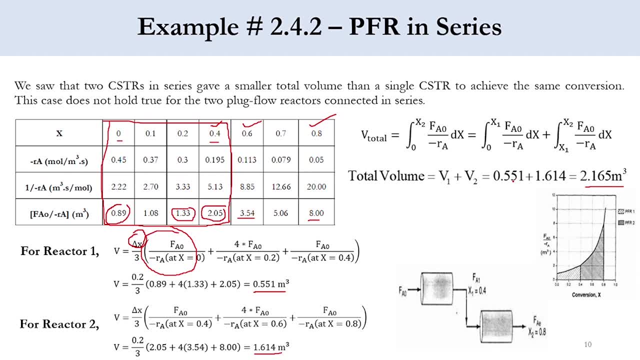 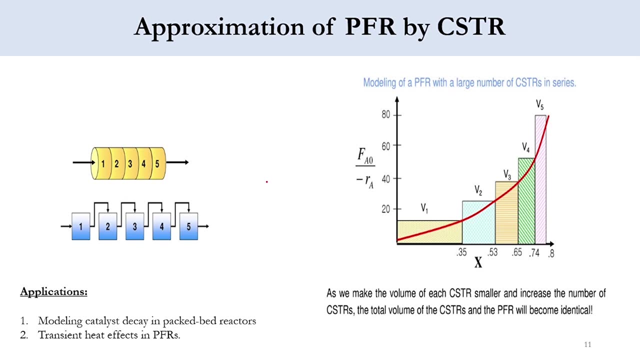 you can say, is because of the nature of the equation, that is, an algebraic equation, that is a differential equation, and also their characteristic as well. so this is the overall example of the reactors in series. and finally, approximation of pfr by cstr: that instead of installing one pfr we can install multiple cstrs and if their volumes 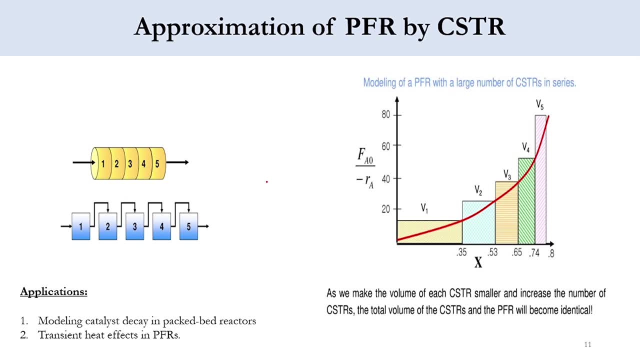 is summed up that will be equal to the pfr modeling of a pfr with a large number of cstrs in series. as we make the volume of each cstr smaller and increase the number of cstr, the total volume of cstrs and the pfrs will become identical, because it represents this area, the area under the. 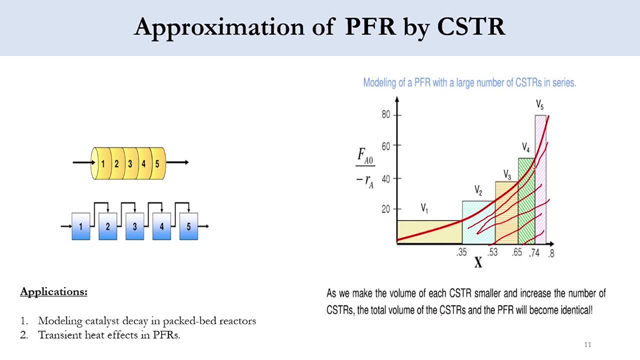 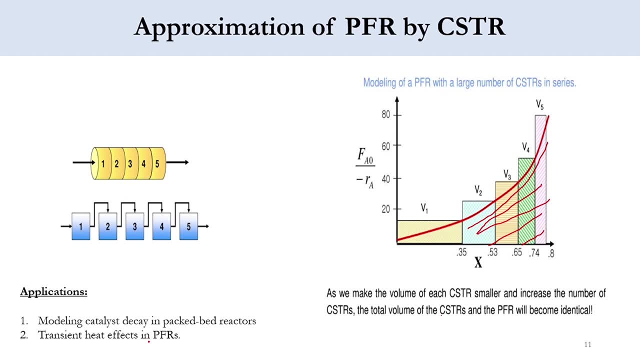 in pack bed vectors and to study transient heat effects in pfr. so that's it from today's lecture. we have seen that how we can connect vectors in series, how will be the equation? for cstr, it will be a different pattern. for pfr it will be a different pattern. we have seen that if we install.